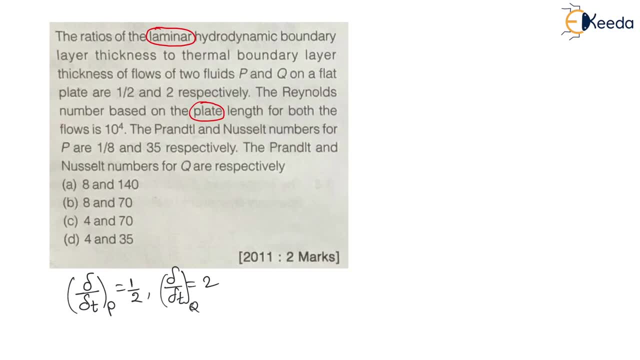 the flows is 10 to the power 4.. Now here, Reynolds number for P is equal to Reynolds. number for Q is equal to 10 to the power 4.. Then the Prandtl and Nusselt number for P are now here. they have given Prandtl number. P are for flow, P, which is 1 by 8. here you can find, and Nusselt. 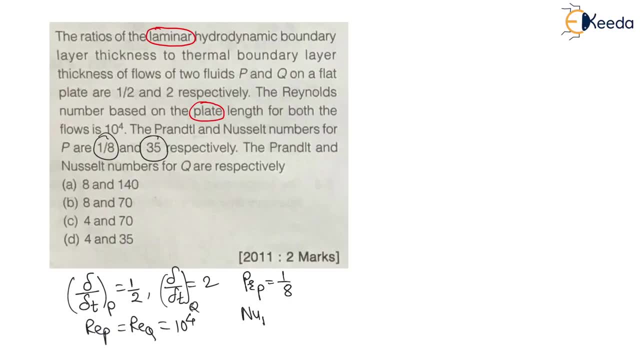 number is 35 for P only And Nusselt number for P is equal to 1 by 2 and for Q is equal. number for p is equal to 35 right respectively. the prontal and nusselt number for q are respectively: 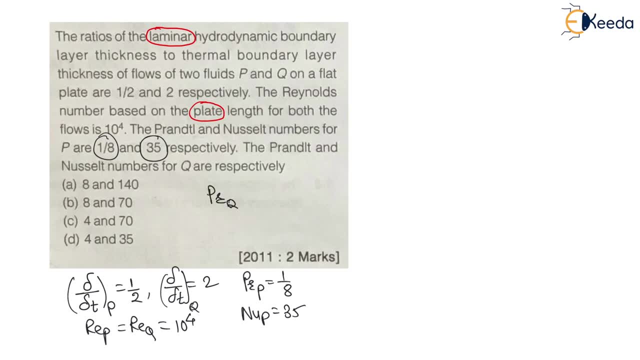 now they are asking: what is the prontal number? first prontal number for q question mark and second nusselt number for q question mark. this is a question right now, my dear students, very, very important relation here for laminar: laminar flow over surface or flow over plate or any. 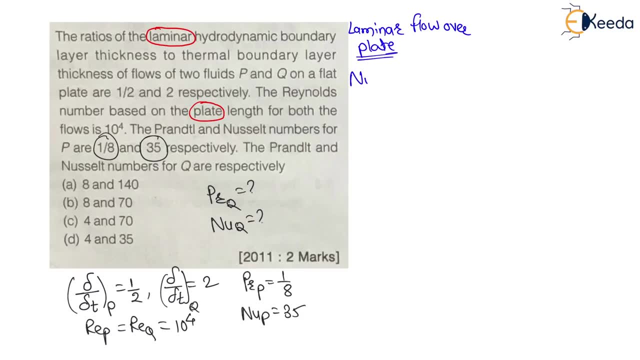 surface. right now we have the relation of nusselt number with renal number and prontal number for such cases. in theory lectures we have seen this relation, that is, nusselt number is directly proportional to renal number power 1 by 2, prontal number, power 1 by 3. this is a relation very, very. 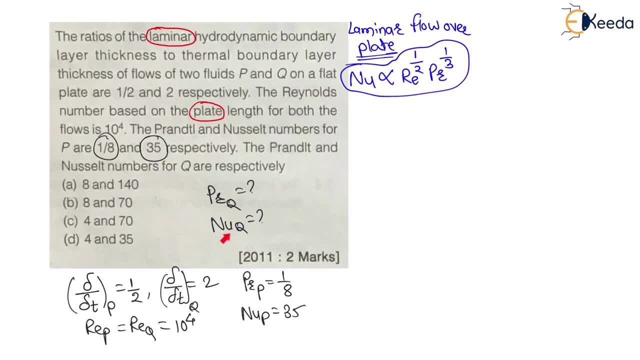 important relation right. with the help of this relation we can find nusselt number of q, right, but before this, let us find prontal number of q. now, my dear students, again we have relation between prontal number and r ratio of hydrodynamic boundary layer thickness and thermal boundary layer thickness, here the 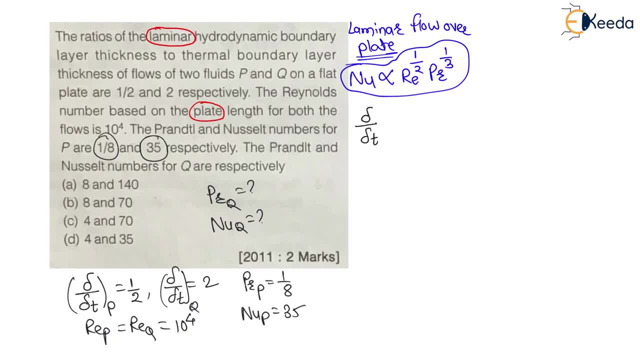 hydrodynamic boundary layer thickness. delta divided by thermal boundary layer thickness. delta t is related with prontal number, is equal to prontal number power, 1 by 3. this is the relation between delta and delta t. now here for p delta. by delta t is given, which is 1 by 2. right here for p delta. 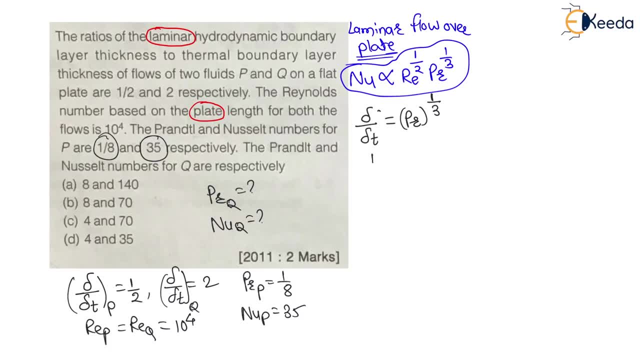 is given, which is 1 by 2. if i use for p 1 by 2 for a p, therefore prontal number for the p power, 1 by 3, if i solve this frontal number for p, i will get- let us solve this, then- frontal. 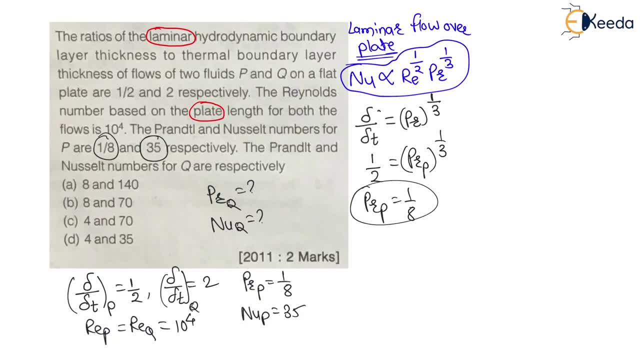 number for p, i will get 1 by 8. but, my dear students, this is given in the question already they have given and there is absolutely no need to provide this frontal number of p, because from this relation we can find frontal number of p. but as they have given, let us forget. 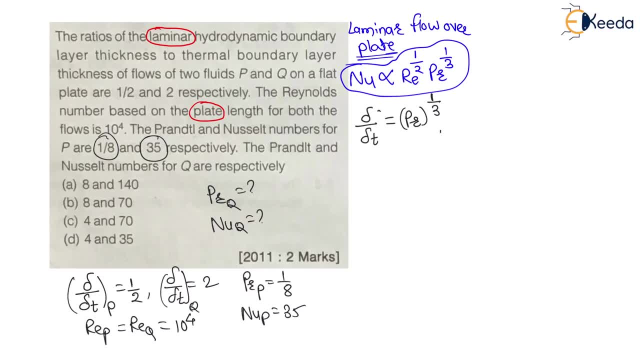 about this, or let us ignore this right again. the same relation i can use for q also. therefore, Therefore, del divided by del t for flow q is equal to frontal number of q raised to 1 by 3.. Therefore, here, hydrodynamic boundary layer thickness divided by thermal boundary layer thickness for q is given 2,. 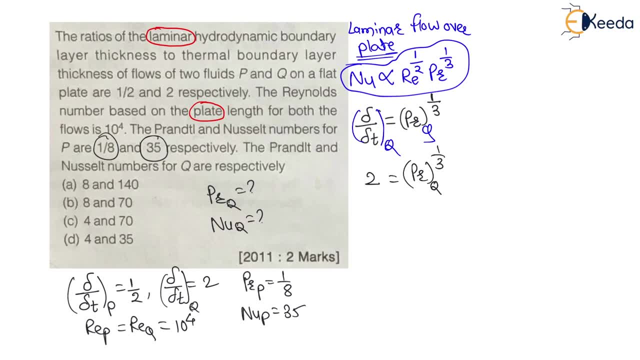 which is equal to frontal number of q, power 1 by 3.. Therefore I can say frontal number of q is equal to 2 power 3, which is equal to 8.. Therefore here frontal number of q is 8.. 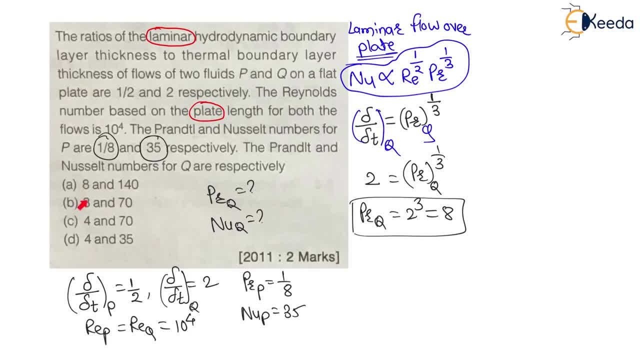 Now look at the option Here. a and b is 8. option c and d is 100% wrong. Therefore we have to select between a and b. Now let us solve for Nusselt number. Now we have Nusselt number relation. 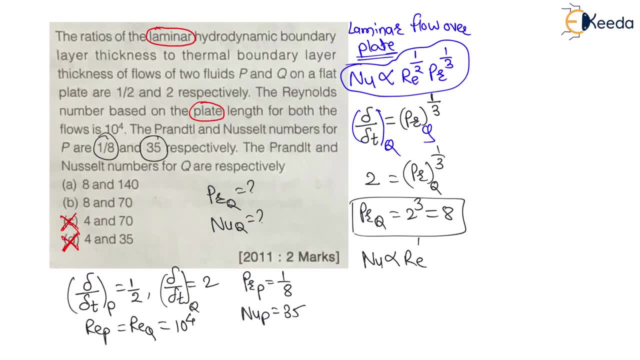 Therefore, here we have relation: Nusselt number is directly proportional to Reynolds number power 1 by 2, frontal number power 1 by 3.. Now, with the help of this relation, if I take ratio of Nusselt number of q to the Nusselt number of p, 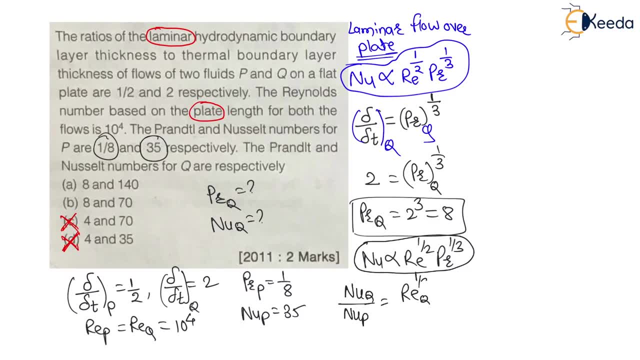 then I will get Reynolds number of q power 1 by 2, frontal number of q power 1 by 3, whole divided by Reynolds. Reynolds number of p power 1 by 2 and frontal number of p power 1 by 3.. 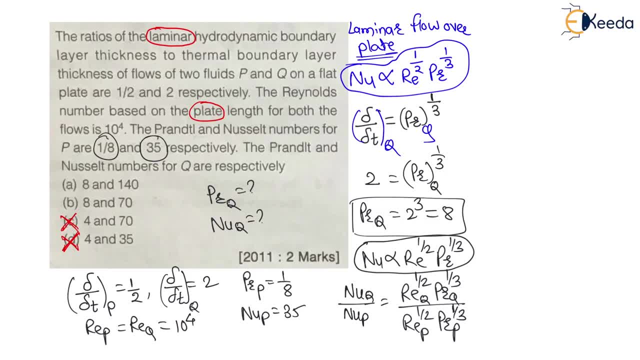 Now, my dear students here, Reynolds number of both flows is same. Therefore, this Reynolds number power 1 by 2 will get cancelled for both flows. Therefore, the resulting equation will become- let us write here: resulting equation. Therefore, my dear students here, the resulting equation becomes: Nusselt number of q divided by Nusselt number of p is equal to: 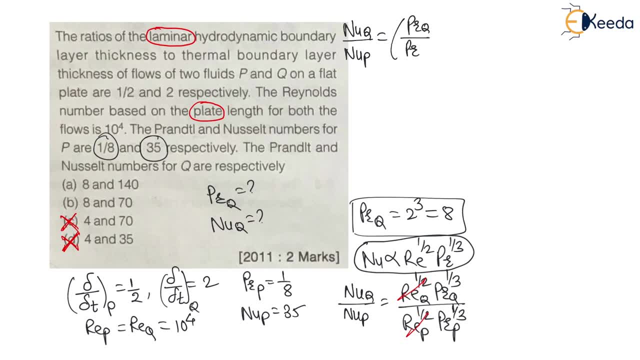 here frontal number of q divided by frontal number of p power, 1 by 3.. Therefore, let us put the values. Therefore, Nusselt number of q is equal to Nusselt number of p, is given 35, right 35 into frontal number of q. 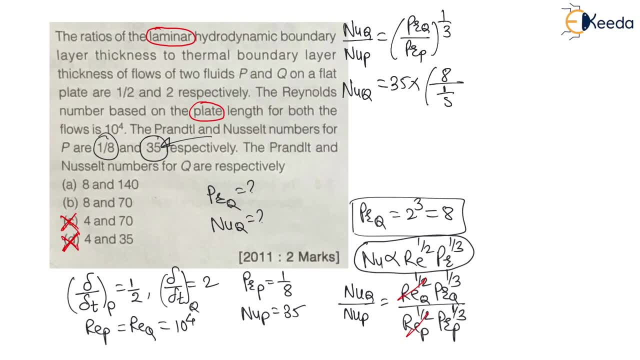 we have calculated as 8, frontal number of p is 1 upon 8, power 1 by 3, right. Therefore, this Nusselt number of q is equal to 35 into 64, power 1 by 3, right.